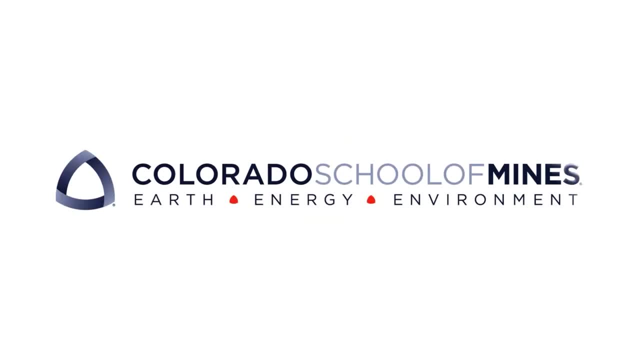 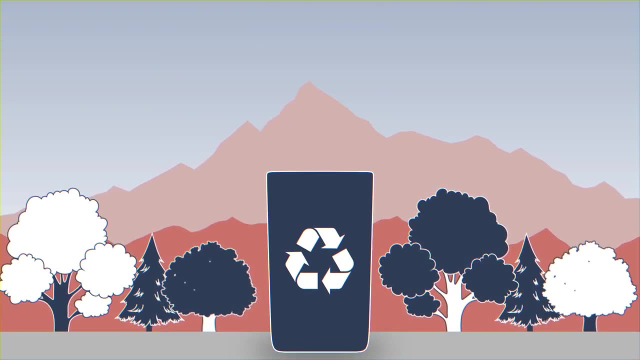 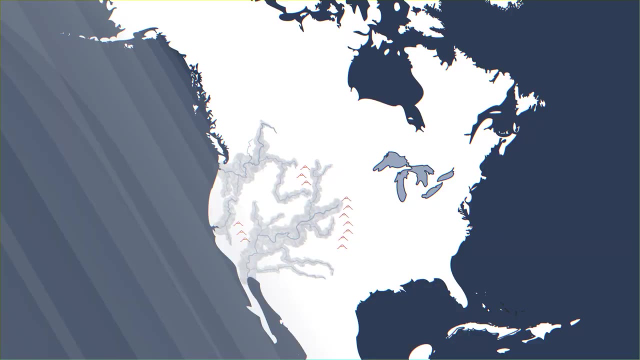 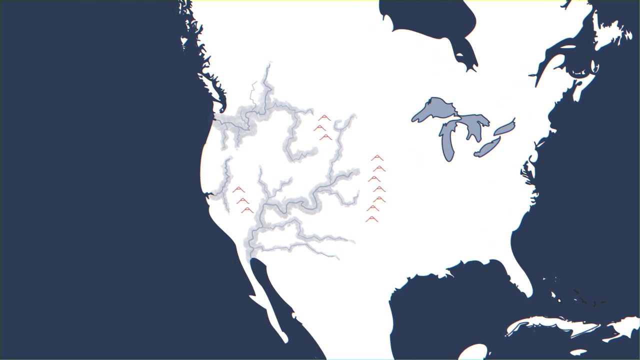 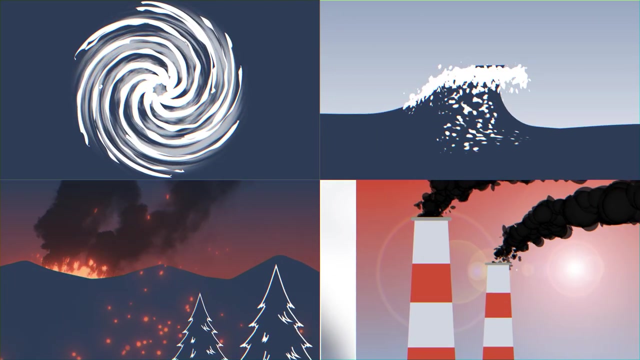 We recycle used plastic bottles, used cardboard boxes and used aluminum cans, But can we recycle our used water? Over the past few years, we've seen massive droughts in the western United States, stressed drinking water supplies, hurricanes, tsunamis, wildfires and other natural disasters, along with human 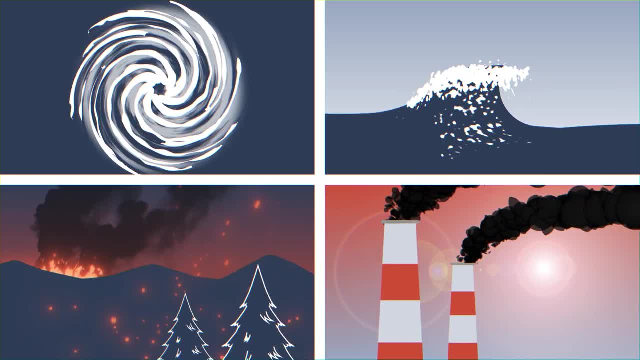 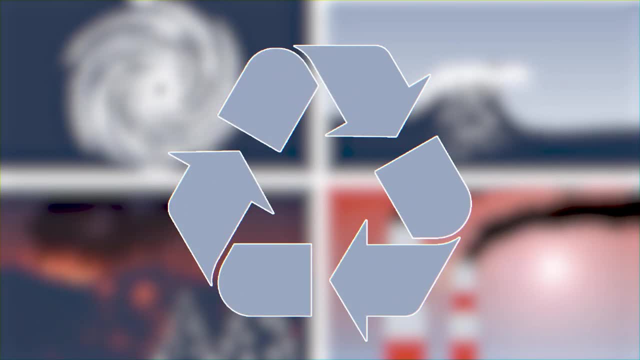 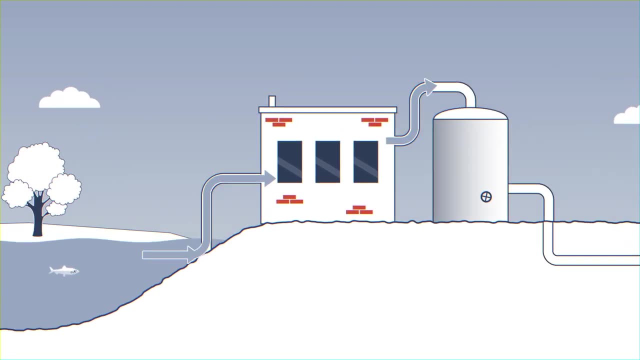 activities often contaminate water supplies around the world. Recycling water for drinking might just hold the key to reducing pressure on critical water supplies. Most cities pull drinking water from a local reservoir. Cities pump and filter the water before it reaches your kitchen tap. When you run your sink or 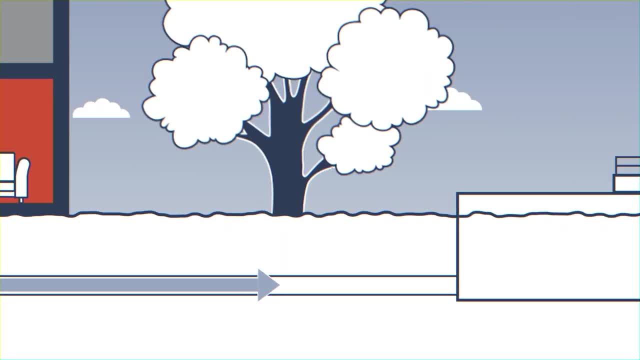 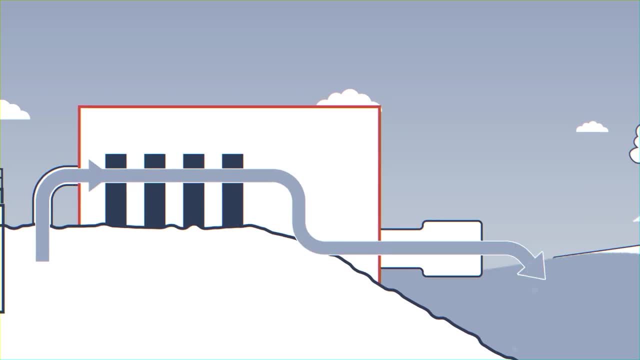 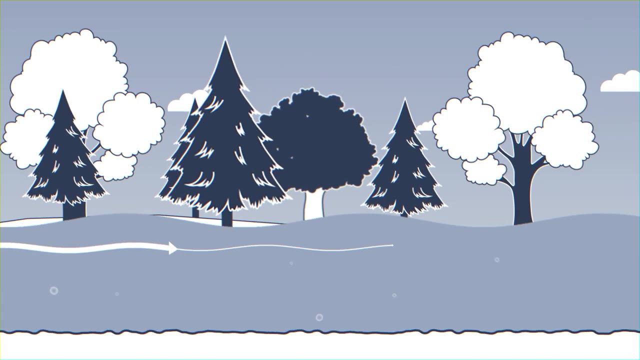 flush the toilet. the used water goes out through your pipes to a wastewater treatment facility that gives it another thorough treatment and filtration before releasing the water out to the local creek or river. The water gets diluted in the environmental buffer flows downstream, receiving a natural treatment. 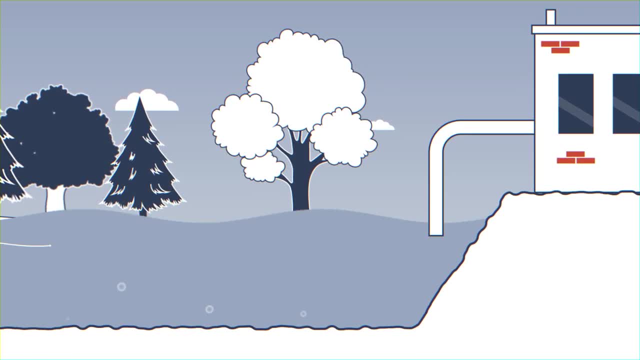 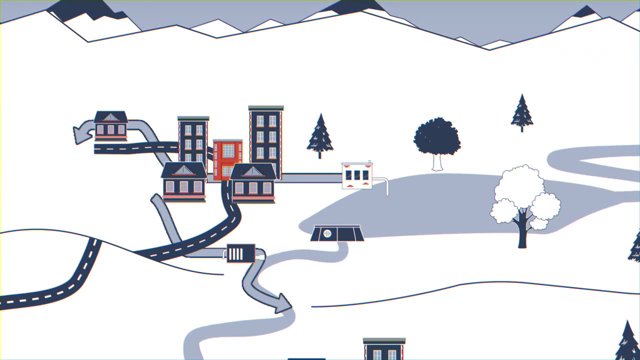 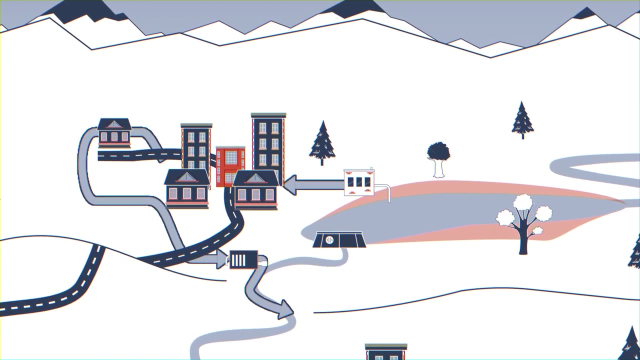 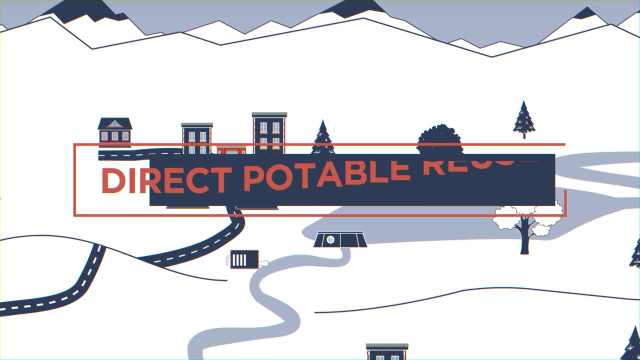 until it reaches the next city using that water supply. This is called indirect potable reuse, and it's often the only way cities access water. However, in a dry year or during a drought, the water supply from the local reservoir runs low, straining water resources. That's where direct potable reuse or DPR systems 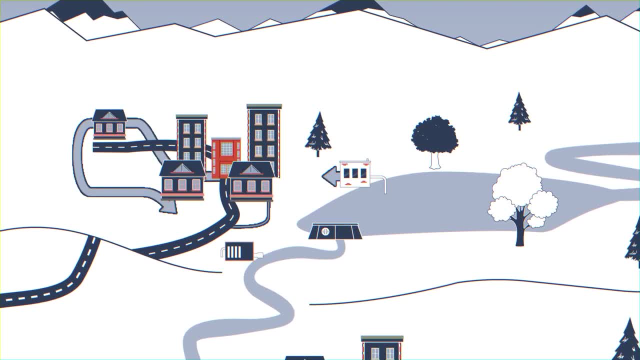 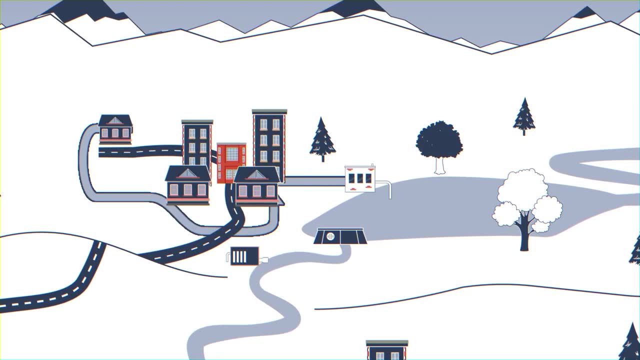 come into play. Rather than drawing water in and pumping it back out with just a single use, DPR systems allow a city to recycle and reuse the used water supply. When you run your sink, take a shower or flush your toilet, you'll see the water. 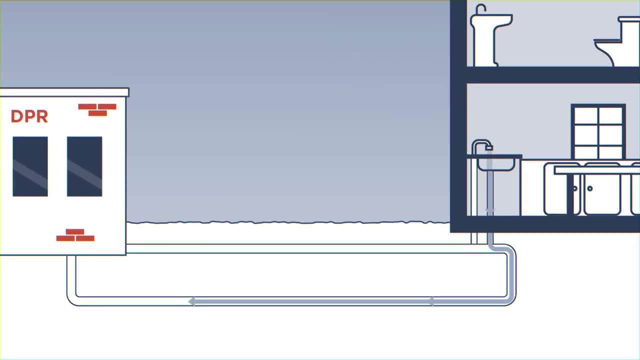 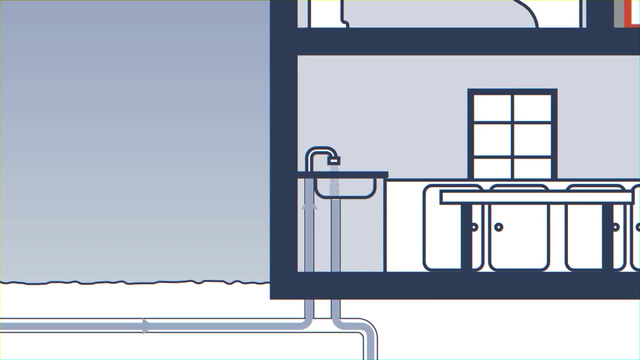 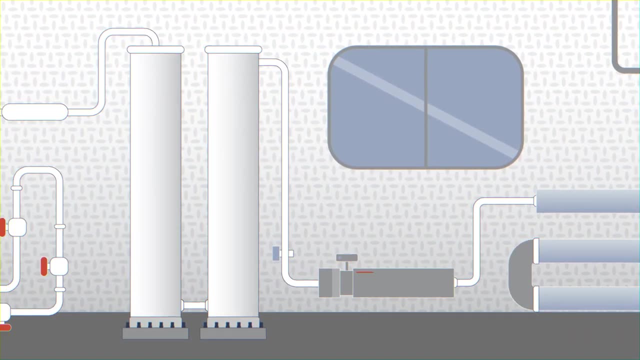 or flush your toilet, the wastewater passes through even more advanced treatment and filtration systems before being routed back into your home for another use, reducing the pressure on reservoirs and water supplies. Researchers at Colorado School of Mines have created a mobile DPR system with a six-step.